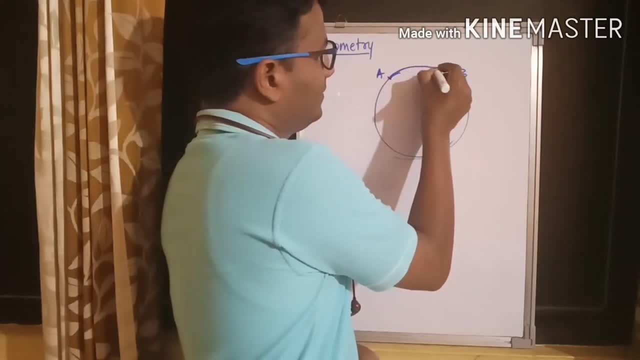 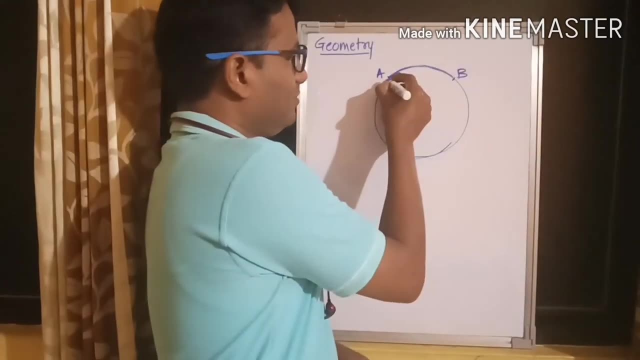 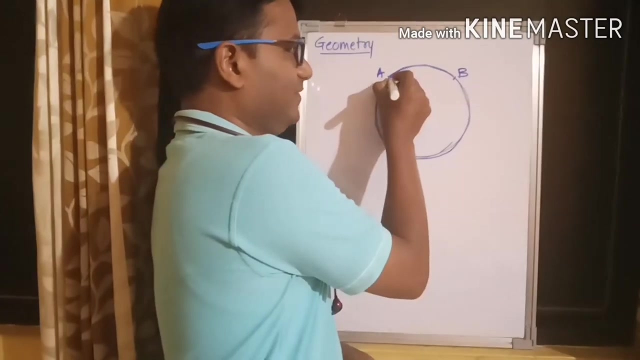 he can walk along the periphery of the well and reach Mr B, like this, or he can walk around by the other side and reach Mr B, or he can jump in the well. he can swim to Mr B Now. 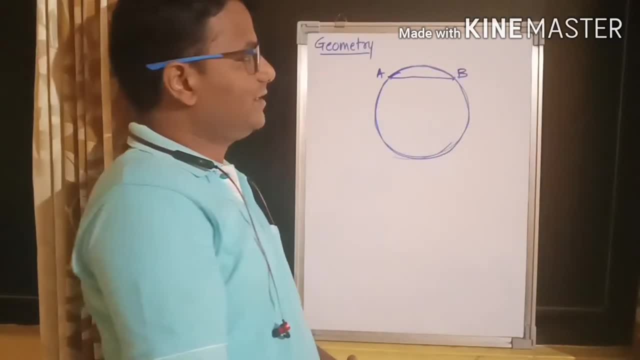 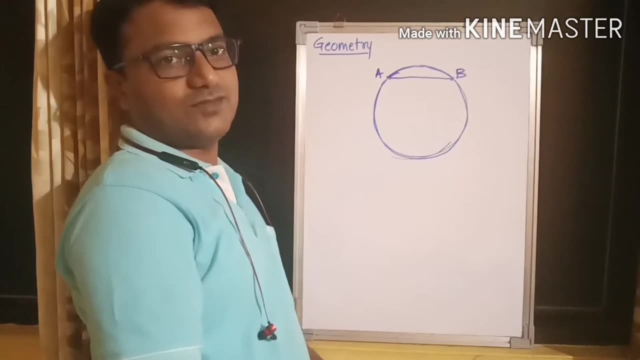 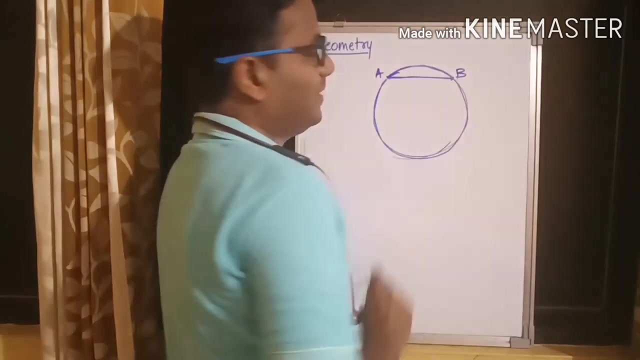 as you see, there are three possible paths he can take to reach Mr B, out of which now let's come across two basic concepts of geometry: chord and arc. You can see, this particular path is a straight line and this particular straight line is connecting two points on. 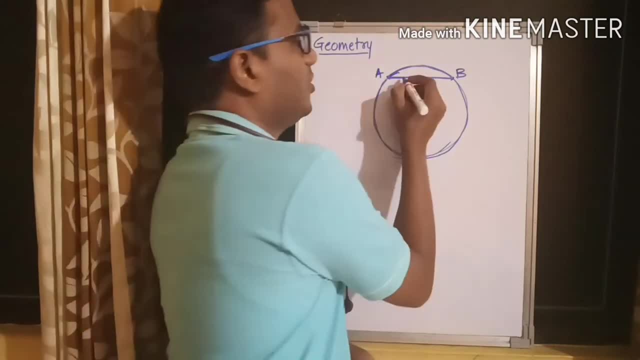 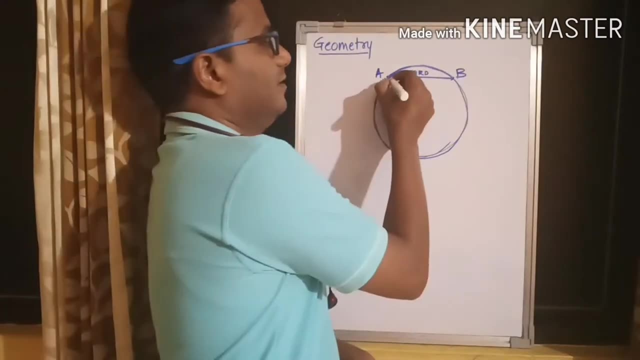 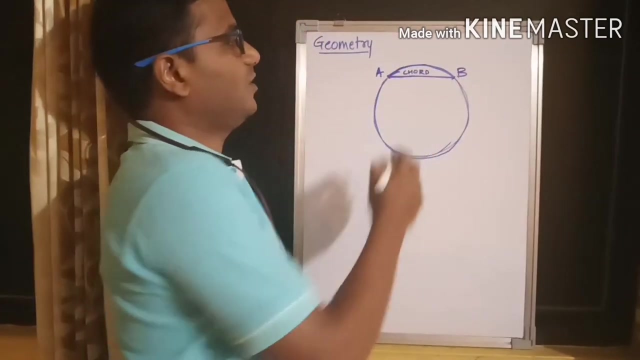 the periphery of the circle, This is called as chord, and the same two points, when joined along the periphery of the circle, are called as chords, And the same two points, when joined along the periphery of the circle, is called as arc. Okay, Now you can see that these 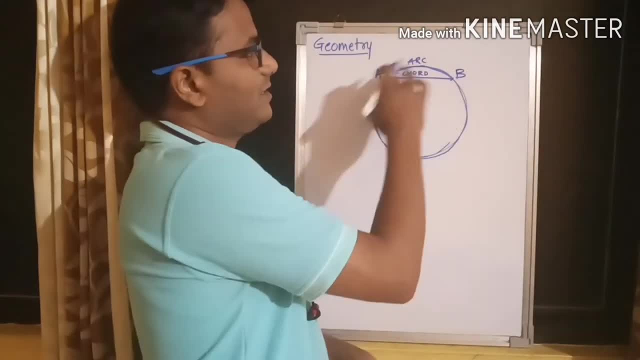 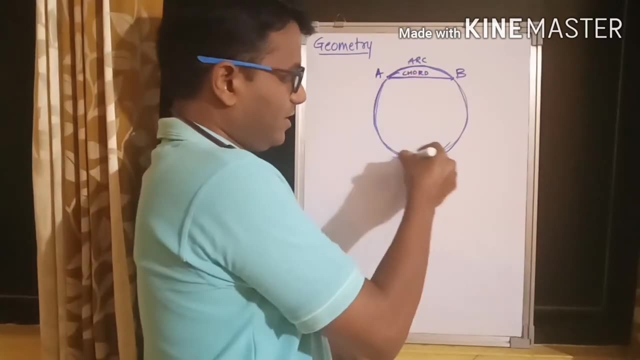 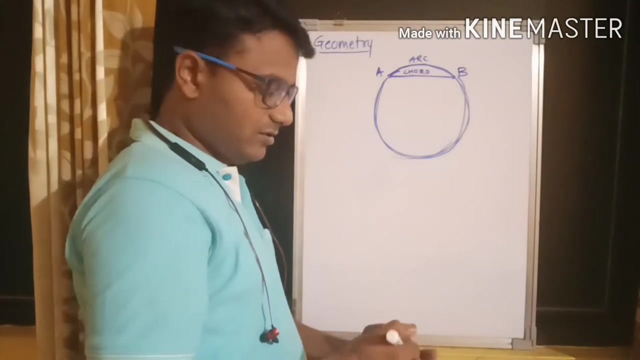 two points are the same but are connected by three different possibilities. Now, this one is also an arc, and this one is also an arc, and this one is quite a long, big curve arc. so right now it will not be a great idea to reach because it would take more. 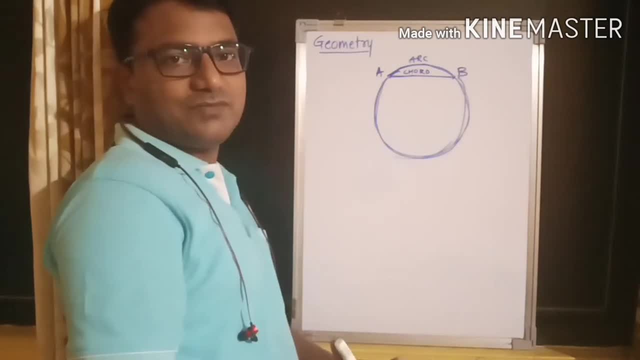 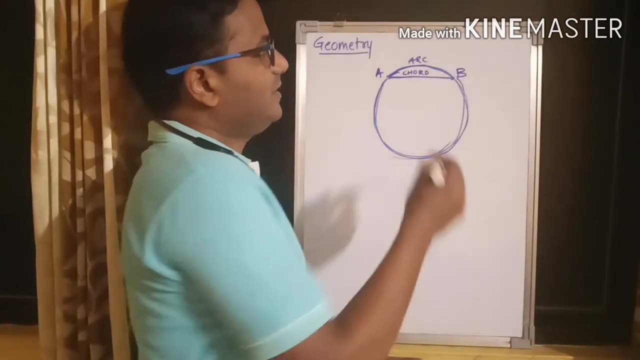 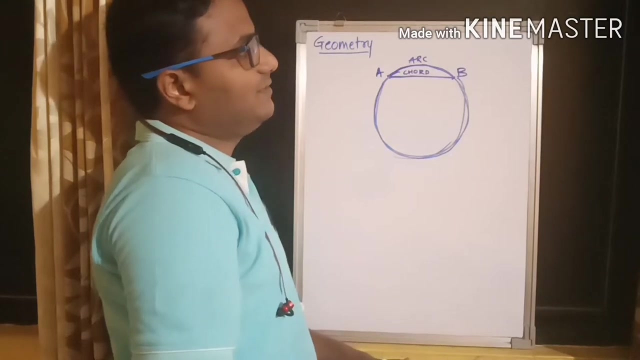 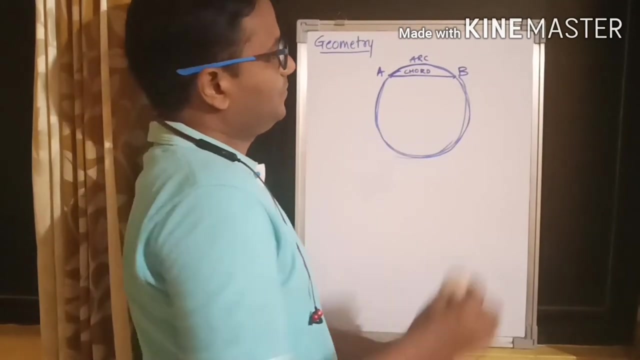 time. so you can see from this picture that the chord is the shortest distance between these two points. okay, so that means the arc length is always bigger than the chord length, correct? now what will be the relation between these two parameters? let's see. now we know, I'll just draw a bigger picture for 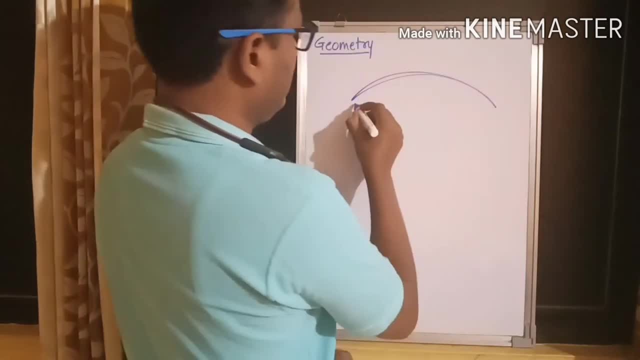 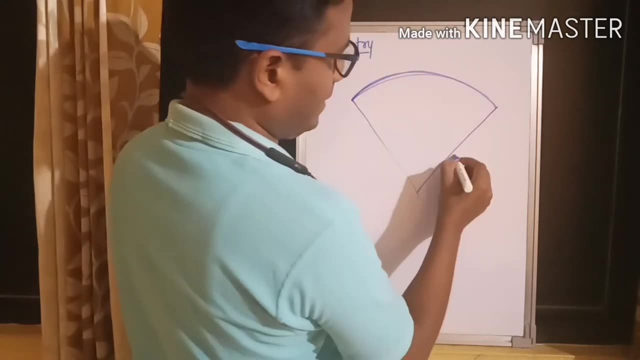 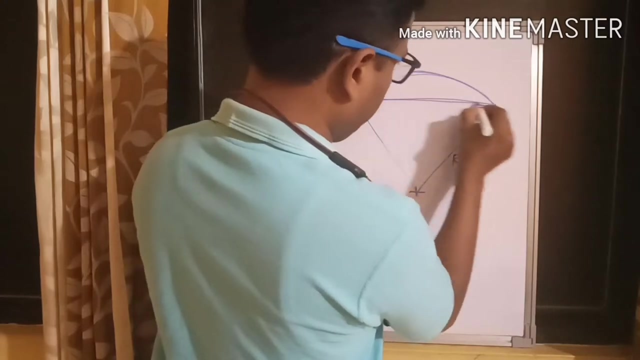 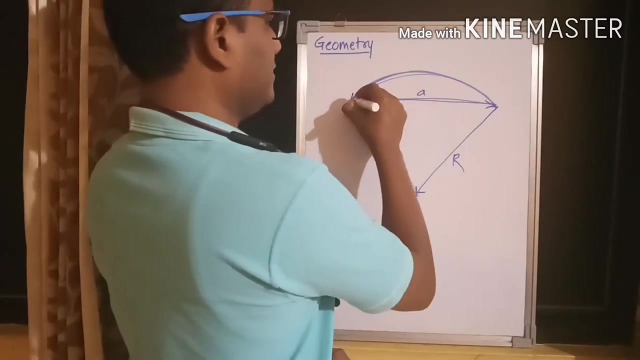 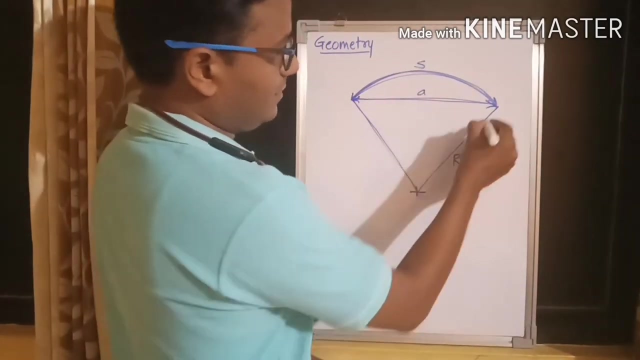 understanding. this is an arc made by a radius R. this is the center of the circle and this one is the chord length. this is the chord length, say I denote chord length by a, and this is the arc length, say I denote by s and the included angle for this chord or this arc. 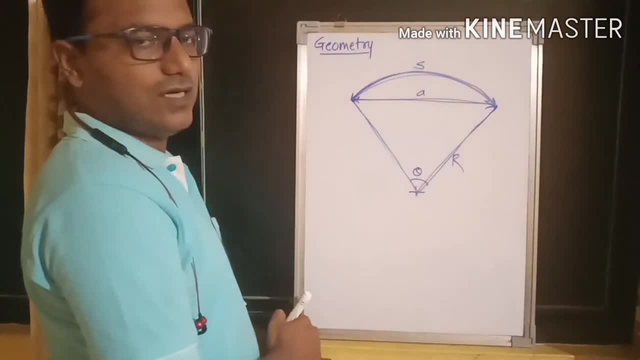 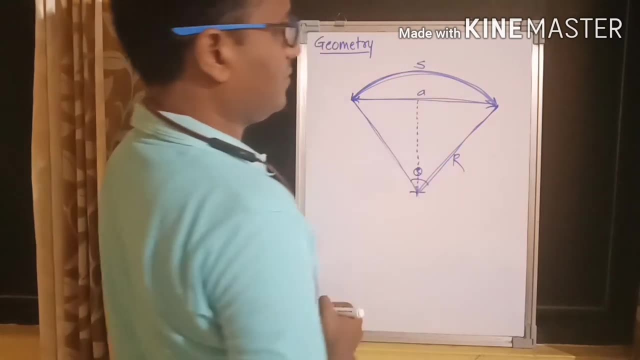 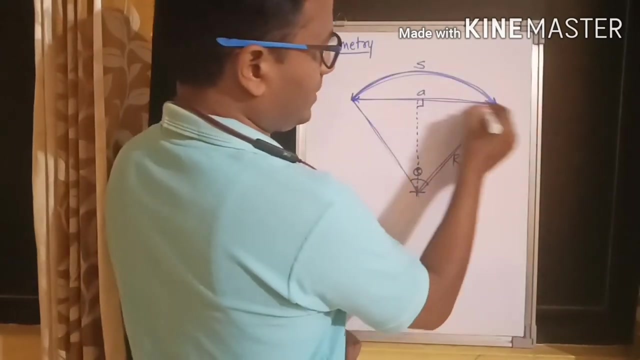 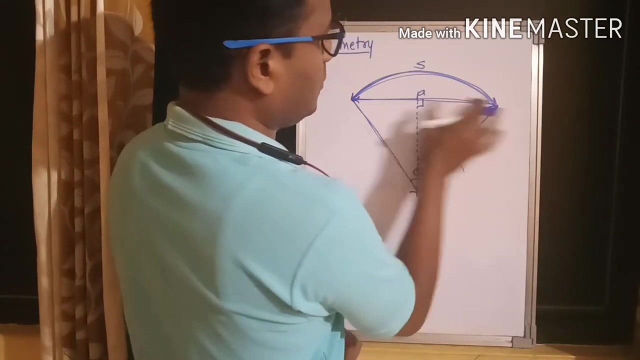 it's a theta. now what I do? I draw a straight line from here, crossing, connecting the chord. now this angle is right spent. now we can see this is a rightidity. this angle is theta by 2. this distance obviously intersect, bisects the chord. so 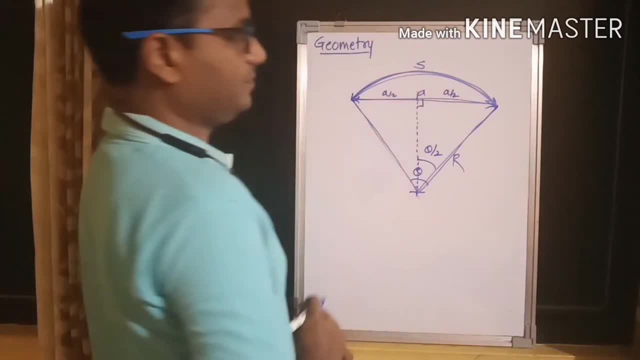 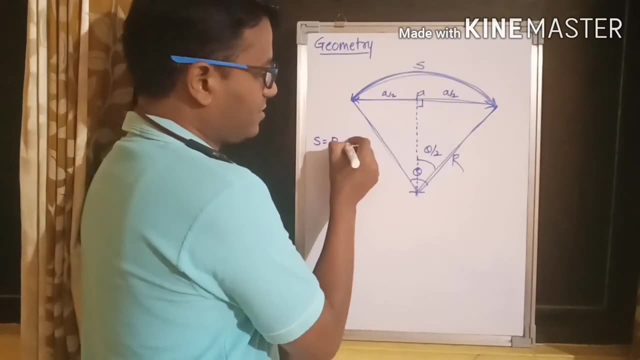 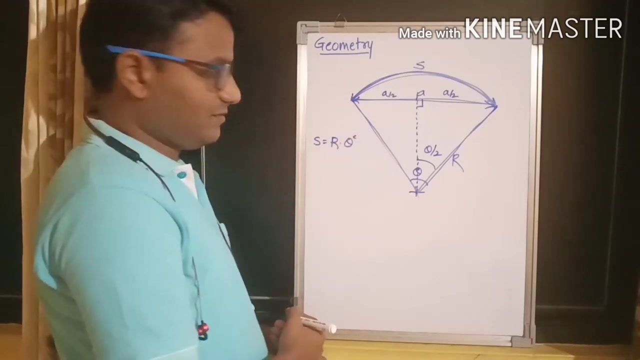 this distance is a by 2. this distance is A by 2. now we know that arc length S is equal to the radius times theta. but remember one thing: this theta is over the one thing, this theta over here is measured in radians. now, if you want to calculate the arc, 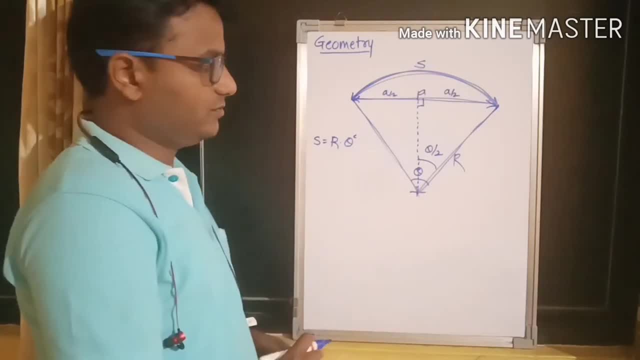 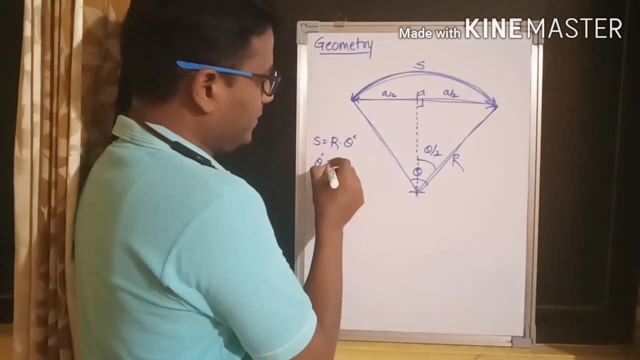 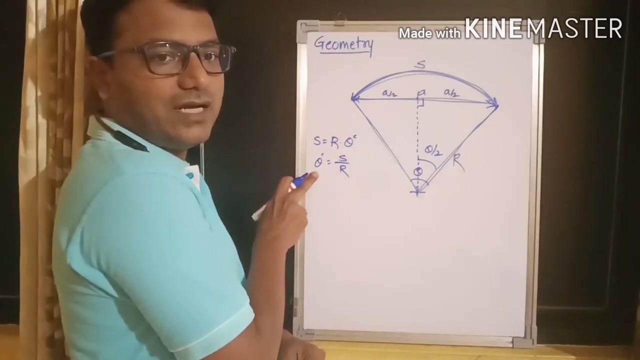 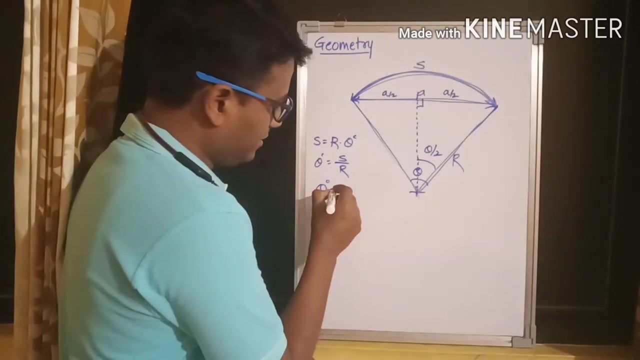 length and you don't know the angle in radians or you have the angle in degrees. so how to convert that into degrees? so theta will be equal to. i take this r on the other side, so it becomes s by r, theta angle in radians. i want to convert this into degrees. so if i want theta in degrees, 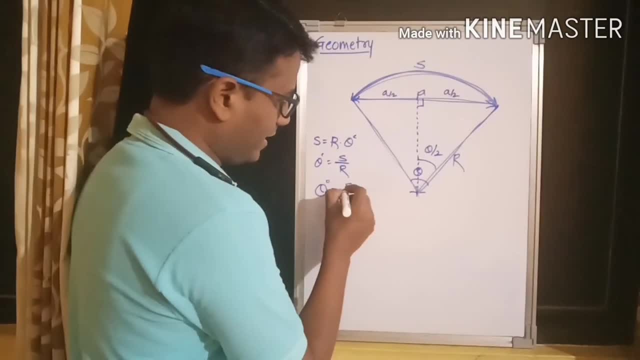 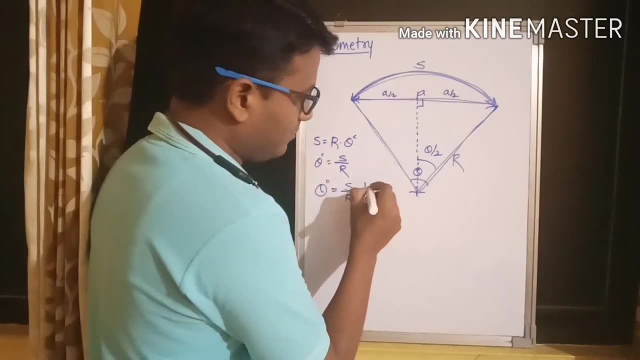 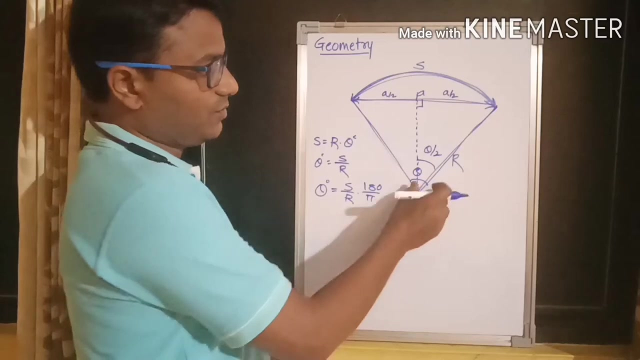 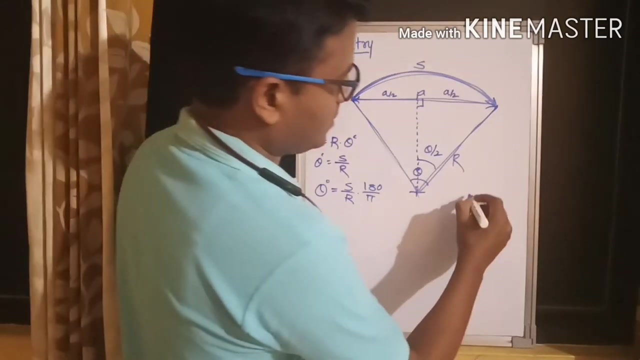 then i have to multiply this value s by r. i. i want to convert radians into degrees, so i have to multiply by 180, correct? now we have the value of theta, the included angle. just consider this particular triangle over here. so it's a right angle triangle. 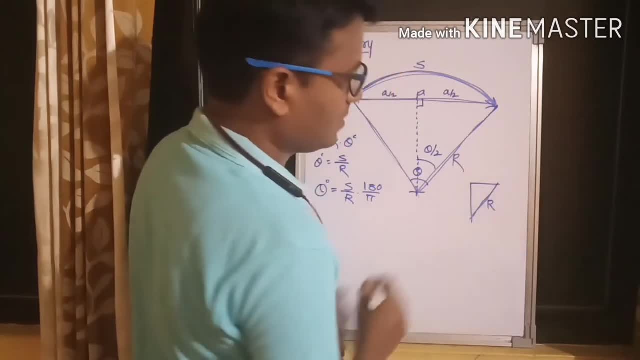 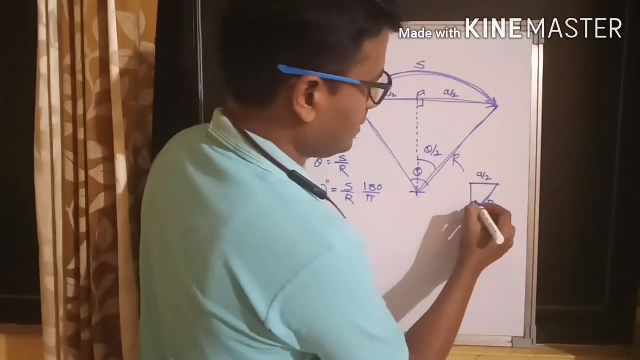 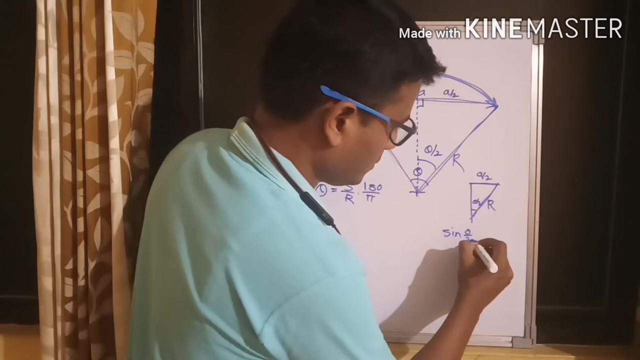 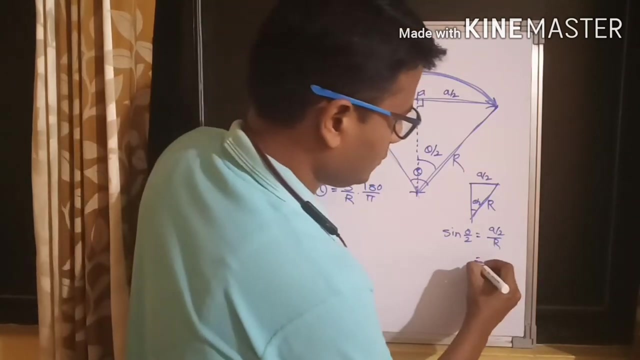 having radius as its one side and one side as a by 2, and this angle is theta by 2. now we know the sine value of theta by 2 will be equal to a by 2 by r, which will be equal to a by 2 r. okay, 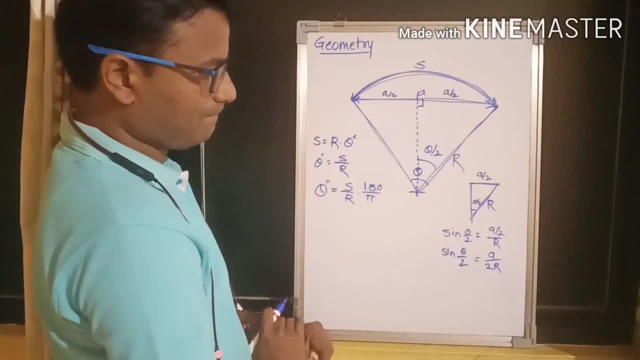 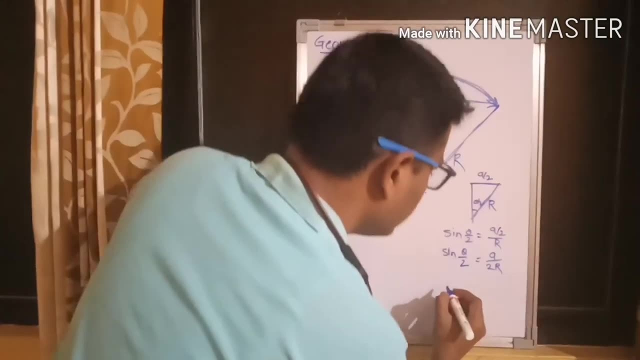 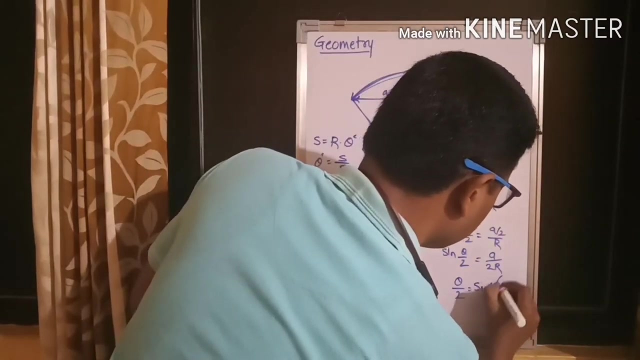 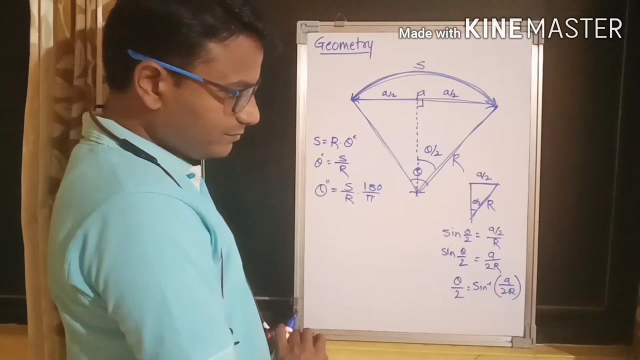 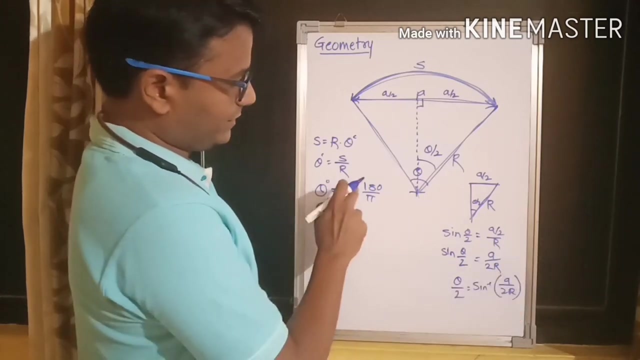 now what we'll do. we'll take inverse of this side, inverse of both the sides, so it will become: theta by 2 will be equal to sine inverse a by 2 r. okay, now what we want to do. we want to calculate, find the relation between a and s over here. 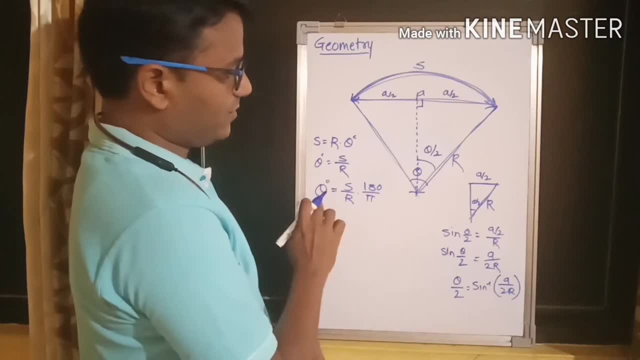 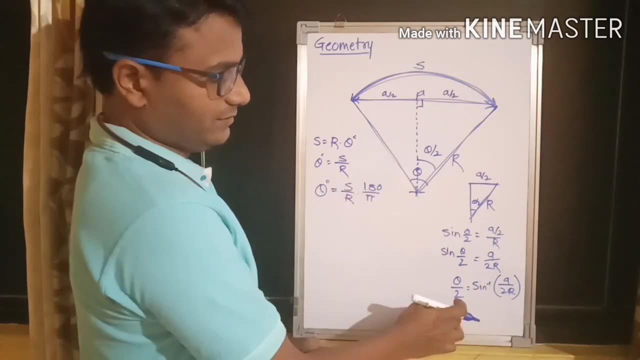 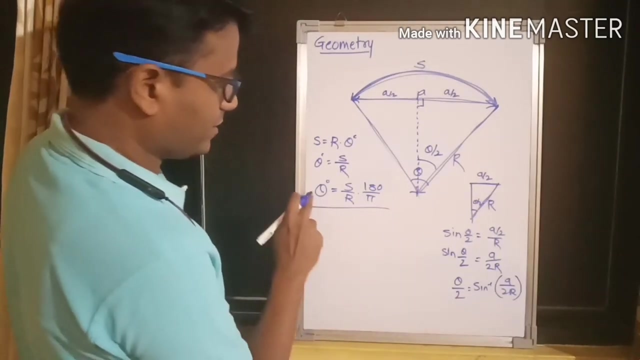 what is common in these two equations? we can see theta is common in these two equations. so what we can do quickly is i can substitute this theta value over here and let's see what happens- this equation over here and substitute this: this is a value over here, so it becomes 1 by 2. on. 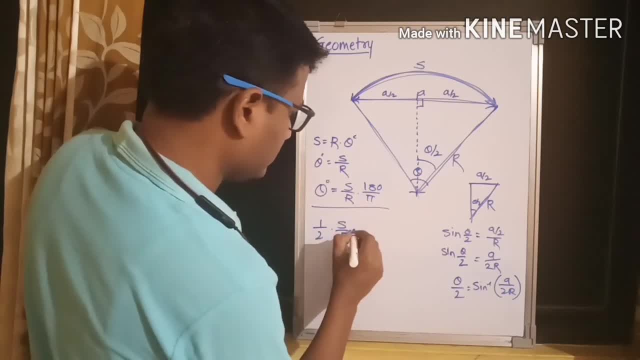 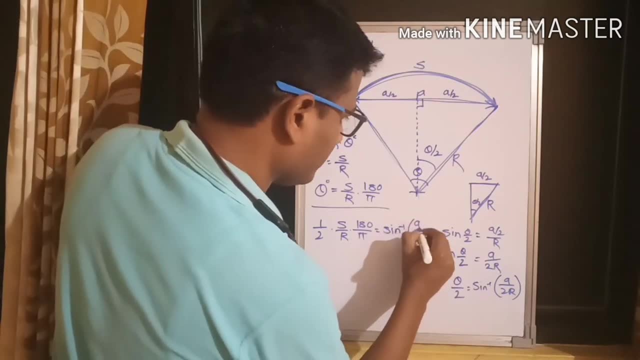 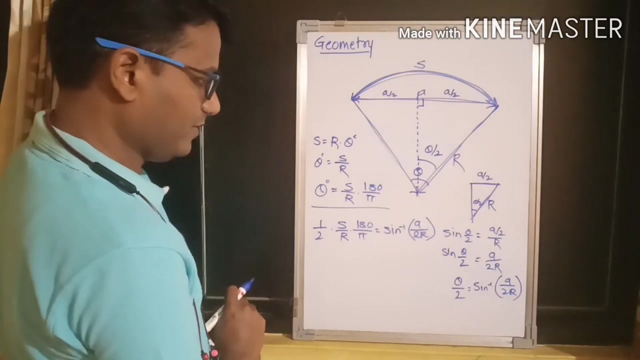 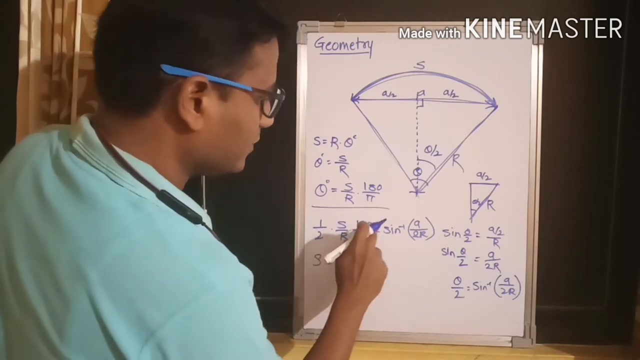 other side, s by r 180 by pi will be equal to sine inverse of a by 2 r. now we're to put this s value on one side, so it becomes: s is equal to this 2 r 180, and pi should go on the right hand side. 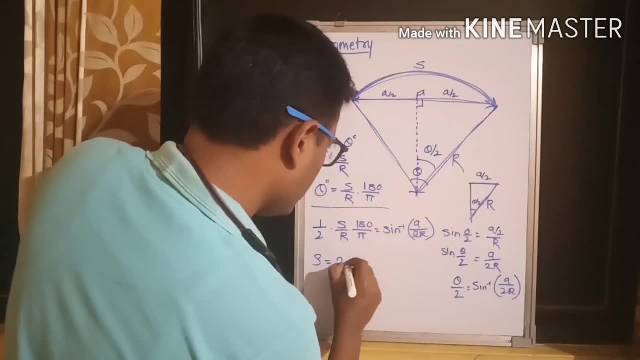 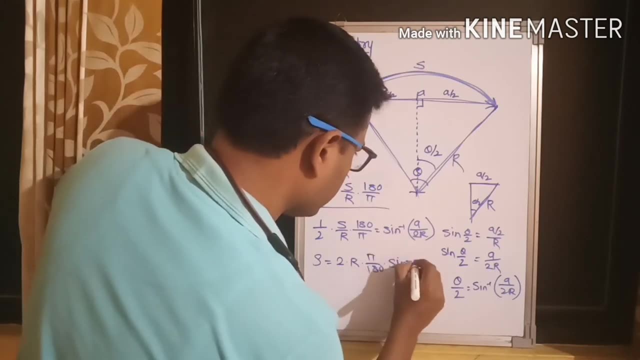 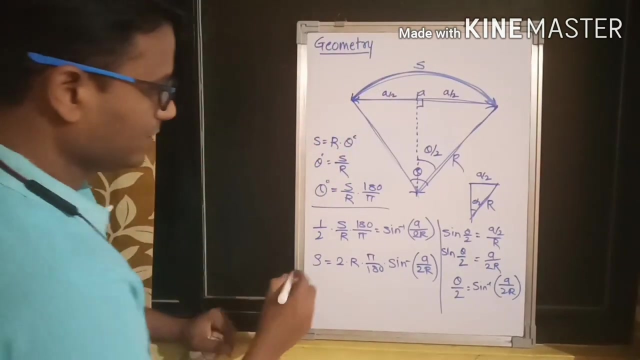 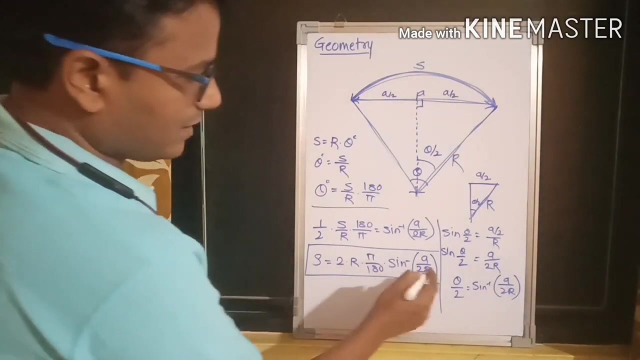 so what will happen over there on right hand side? 2 r pi by 180 into sine inverse a by 2 r, correct? so this gives us the final equation, the relationship between the arc length and the chord length. you can see just. it's easy to. 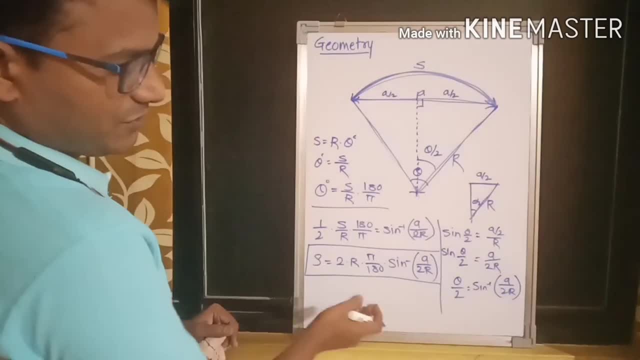 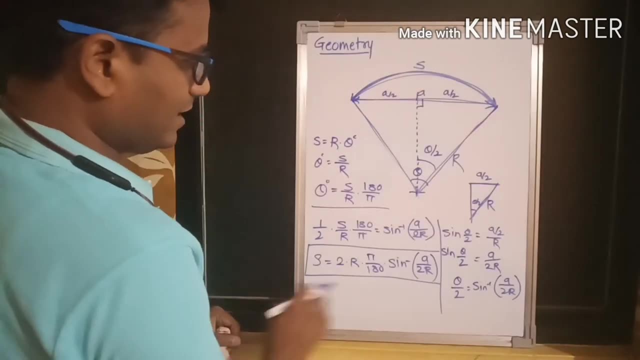 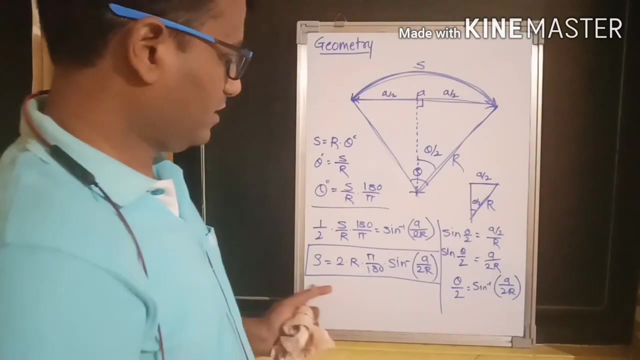 remember this: pi by 180 is because of the conversion of radians into degrees and sine inverse, due to the trigonometry, and 2 r because of the radius. so this is a simple equation which can give you the relationship between arc length and chord length. if you see this,